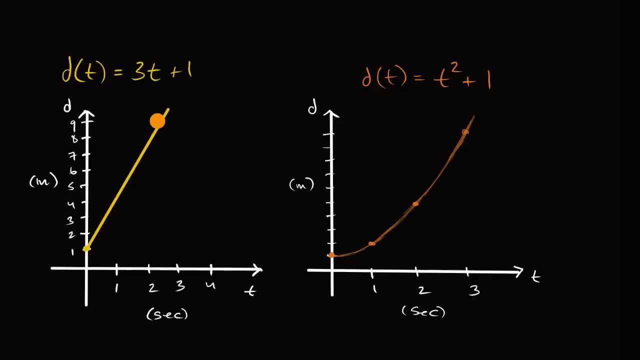 And you can see the graph of how distance is changing as a function of time. here is a line And, just as a review from algebra, the rate of change of a line we refer to as the slope of a line, And we can figure it out. 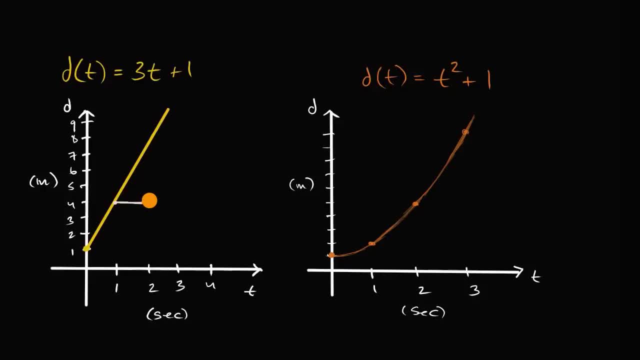 We can figure out well, for any change in time, what is our change in distance. And so in this situation, if we're going from time equal one to time equal two, our change in time delta t is equal to one. 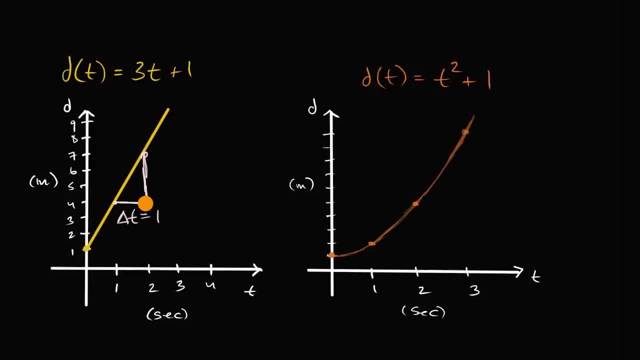 And what is our change in distance We go from? distance is equal to four meters at time, equals one, to distance is seven meters at time, equal two. And so our change in distance here is equal to three. And if we wanna put our units, 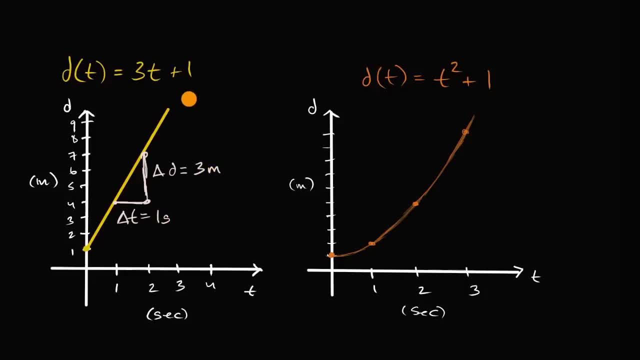 that's three meters for every one second in time. And so our slope would be our change in our vertical, divided by our change in our horizontal, which would be change in d delta d over delta t, which is equal to three over one. 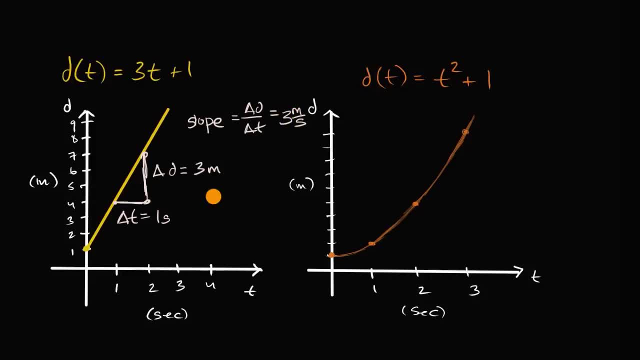 or we could just write that as three meters per second And you might recognize this as a rate. If you're thinking about your change in distance over change in time, this rate right over here is going to be your speed. This is all a review of what you've seen before. 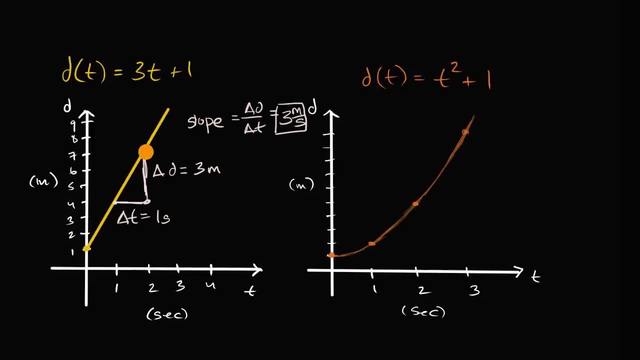 And what's interesting about a line or, if we're talking about a linear function, is that your rate does not change at any point. The slope of this line between any two points is always going to be three, But what's interesting about this function on the right? 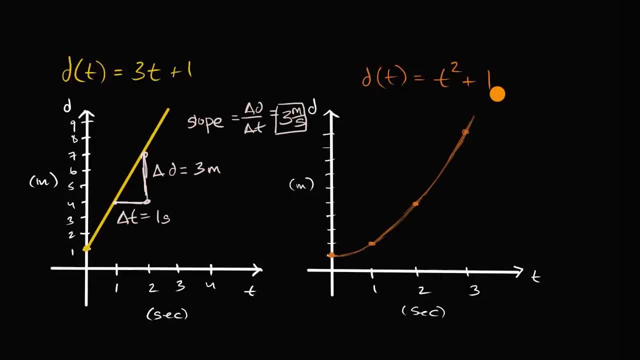 is. that is not true. Our rate of change is constantly changing And we're going to study that in a lot more depth when we get to differential calculus And really this video is a little bit of a foundational primer For that future state when we learn. 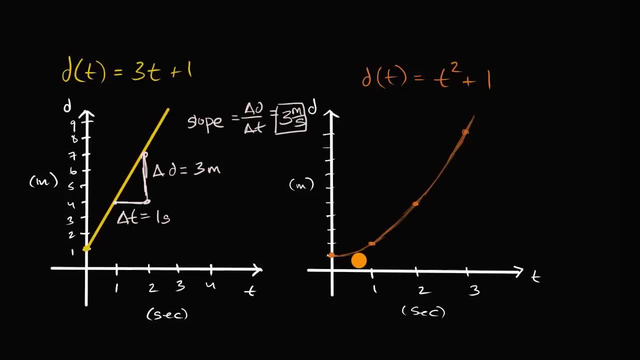 about differential calculus, And the thing to appreciate here is: think about the instantaneous rate of change someplace, So, let's say, right over there. If you were to think about the slope of a line that just barely touches this graph, it might look something like that: 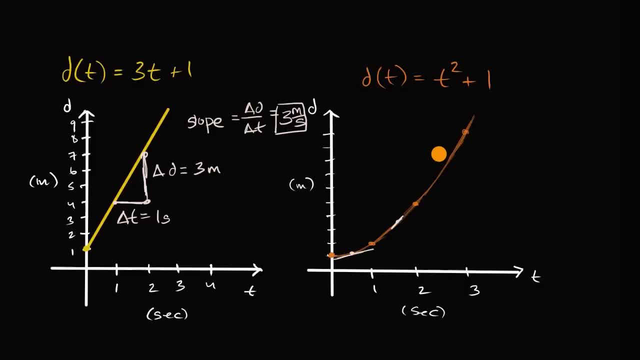 the slope of a tangent line, And then right over here it looks like it's a little bit steeper. And then over here it looks like it's a little bit steeper. So it looks like your rate of change is increasing as t increases. 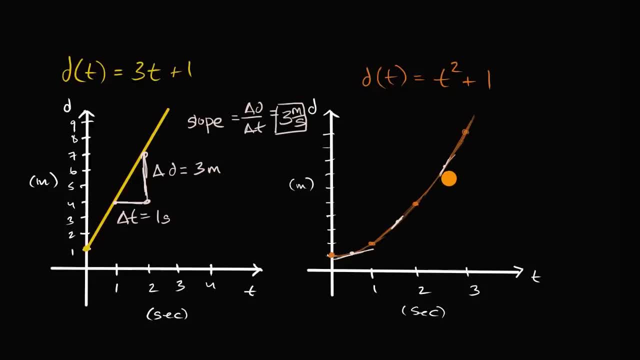 As I mentioned, we will build the tools to later think about instantaneous rates of change, but what we can start to think about is an average rate of change. Average rate of change And the way that we think about our average rate of change is we use the same tools that we first learned in algebra. 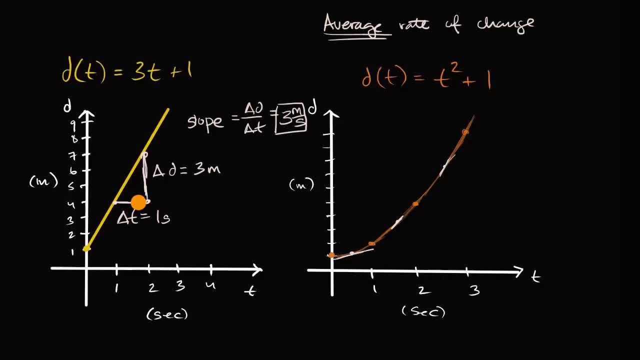 We think about slopes of secant lines. What is a secant line? Well, we talk about this in geometry: That a secant is something that intersects a curve in two points. So let's say that there's a line that intersects. 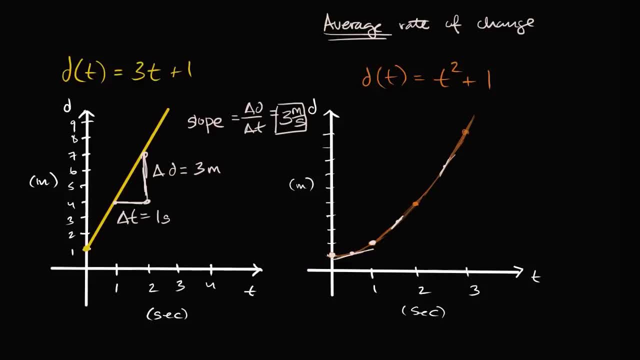 at t equals zero and t equals one, And so let me draw that line. I'll draw it in orange. So this right over here is a secant line, And you could view the slope of the secant line as the average rate of change from t equals zero. 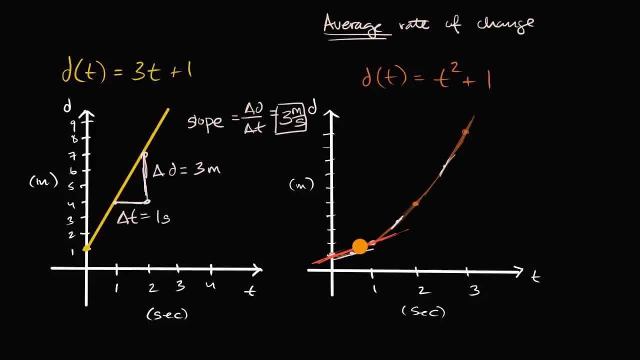 to t equals one. Well, what is that average rate of change going to be? Well, the slope of our secant line is going to be our change in distance divided by our change in time, which is going to be equal to well, our change in time. 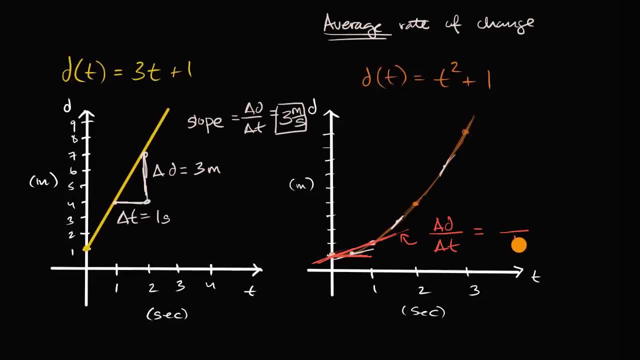 which is going to be equal to well, our change in time, which is going to be equal to well. our change in time is one secant one. I'll put the units here. one secant is one secant one. I'll put the units here. one secant. 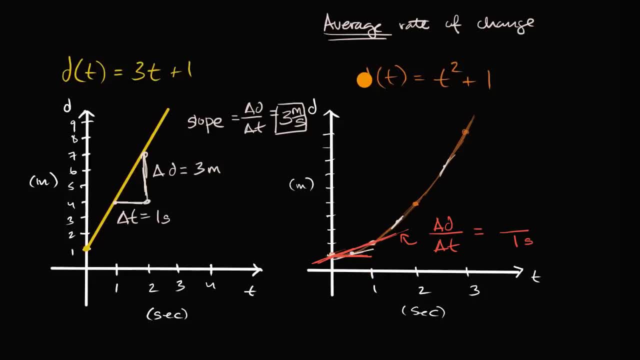 And what is our change in distance? At t equals zero or d of zero is one and d of one is two. So our distance has increased by one meter. So we've gone one meter in one secant, Or we could say that our average rate of change 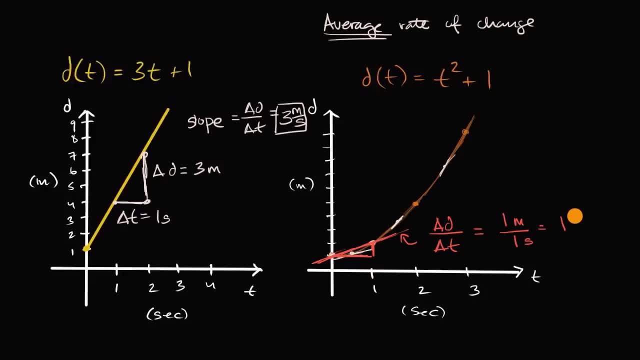 over that. first secant from t equals zero to t equals one is one meter per secant. But let's think about what it is if we're going from t equals two to t equals three. Well, once again we can look at this secant line. 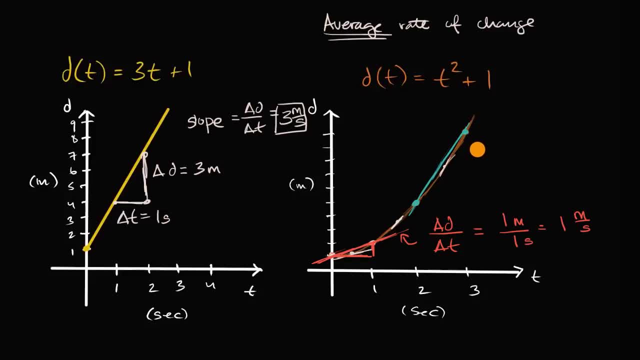 and we can figure out its slope. So this the slope here which you could also use: the average rate of change from t equals two to t equals three. We, as I already mentioned, the rate of change seems to be constantly changing. 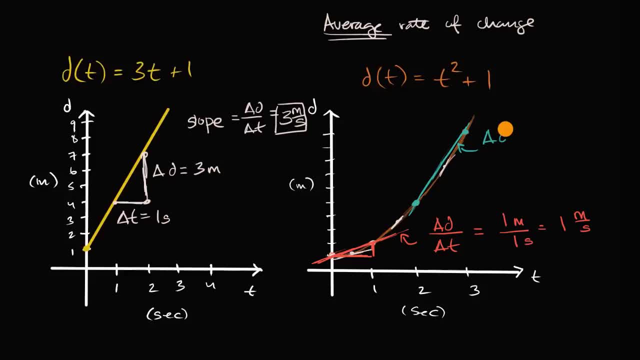 but we can think about the average rate of change, And so that's going to be our change in distance over our change in time, which is going to be equal to when t is equal to two over t equals three. our distance is equal to five. 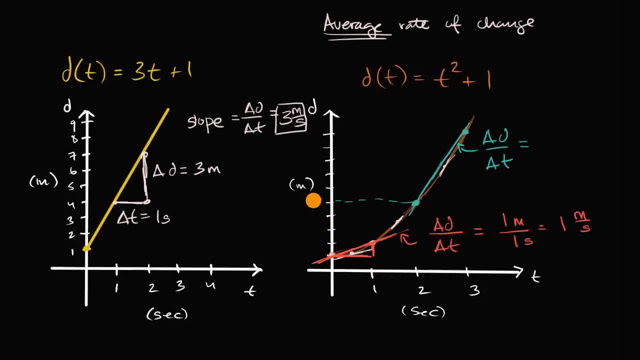 So one, two, three, four, five, So that's five right over there. And when t is equal to three, our distance is equal to 10.. Six, seven, eight, nine, 10.. So that is 10 right over there. 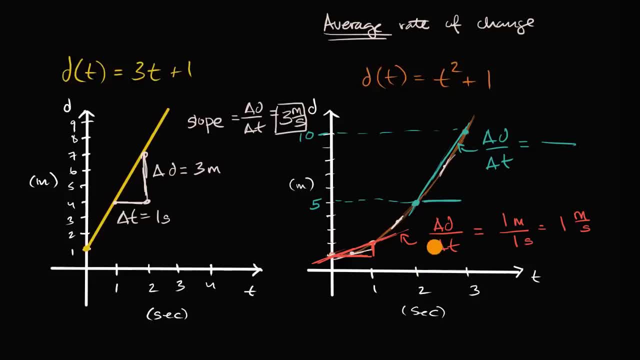 So our change in time? that's pretty straightforward. We've just gone forward one secant, so that's one secant, And then our change in distance- right over here we go from five meters to 10 meters- is five meters. 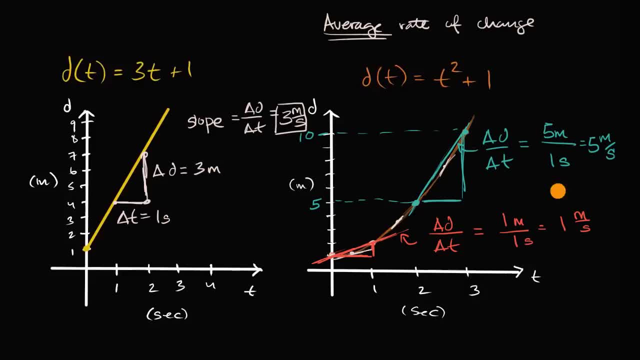 So this is equal to five, So that's five meters per second, And so this makes it very clear that our average rate of change has changed from t equals zero to t equals one to t equals two to t equals three. Our average rate of change is higher. 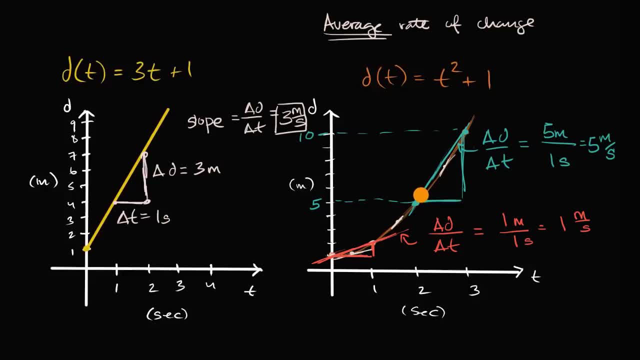 on this second interval than on this first one. And, as you can imagine, something very interesting to think about is what if you were to take the slope of the secant line of closer and closer points? Well then, you would get closer and closer. 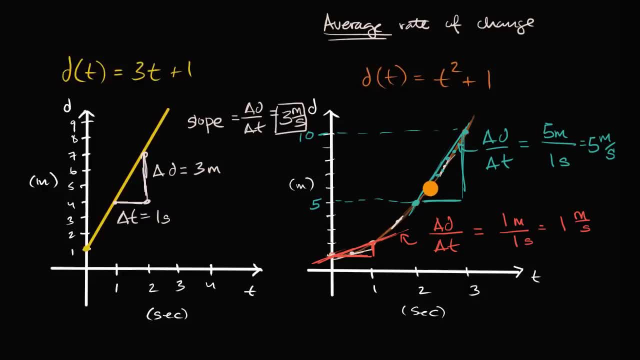 to approximating that slope of the tangent line, And that's actually what we will do when we get to calculus. Hi there, I am Abhay Gadia, your instructor for the course. In this video, we will learn how to create butterfly chart in Excel. This chart is also known as pyramid chart or tornado chart, and so on. This chart is mostly presented where you have two divisions or categories with few common parameters. 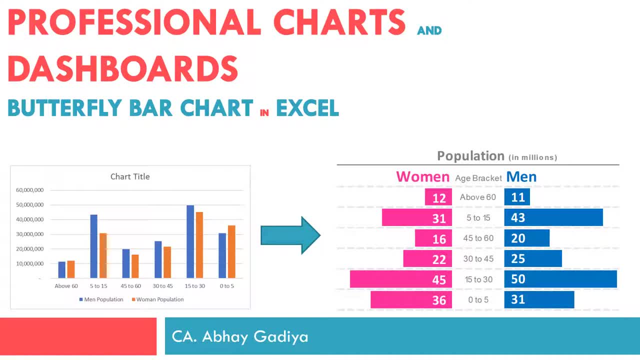 Instead of showing simple vertical or horizontal bar charts side by side, this chart shows diverging horizontal bar charts from the center. There are two approaches to create this chart inside Excel. First one is using data bars from conditional formatting, which we will be seeing in this video.